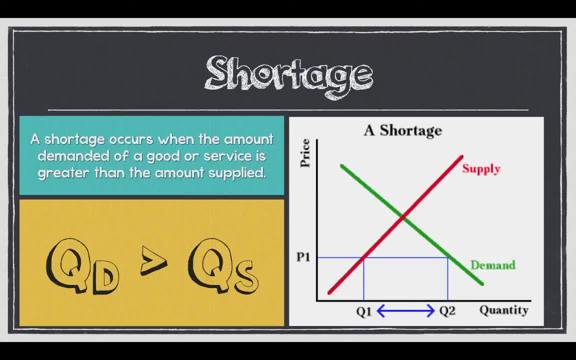 And that distance between the two is the size of the shortage that we're going to occur. Right, The price that a producer is willing to produce is at our Q1. The price that we are willing to purchase is at Q2.. We are willing to purchase more than is. 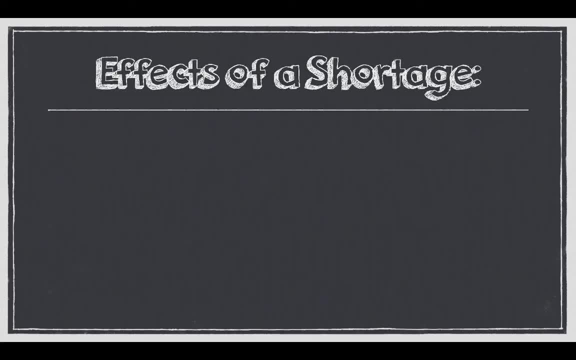 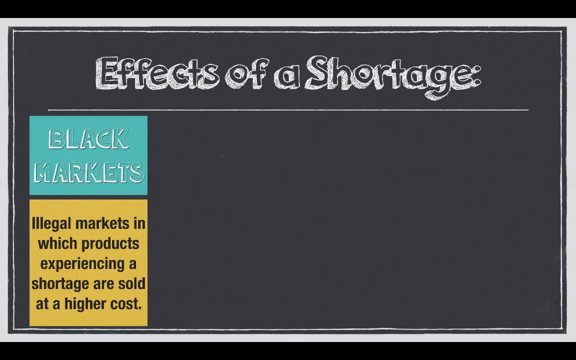 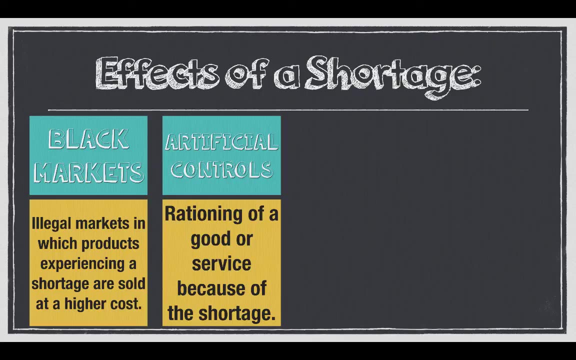 Therefore, we have what's known as our shortage. Moving forward, we see the effects of a shortage. might see black markets pop up like concert tickets selling for two, three times the price, Artificial controls like rationing- Think of rations that we have to go through for watering our plants or getting gas in the 70s, whatever it might be. 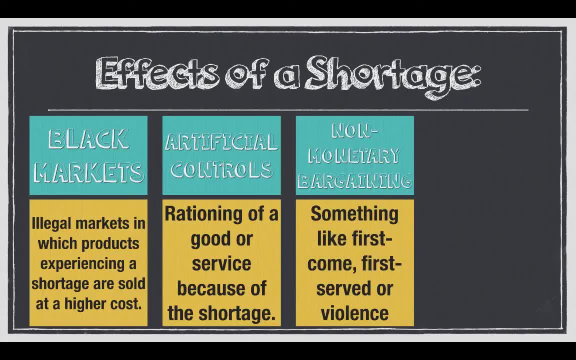 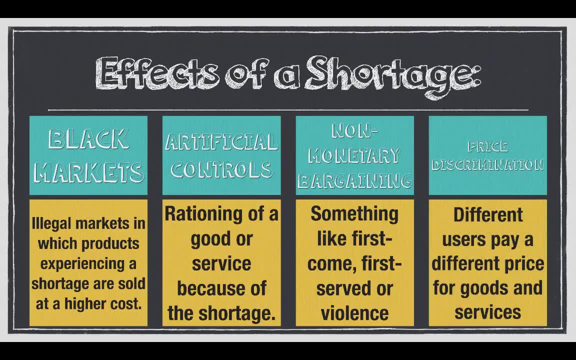 Right. We see non-monetary bargaining, such as first come, first serve or violence in order to get what we want. And, last but not least, we see price discrimination, where prices paid by different users depend on the amount of money that the user has. 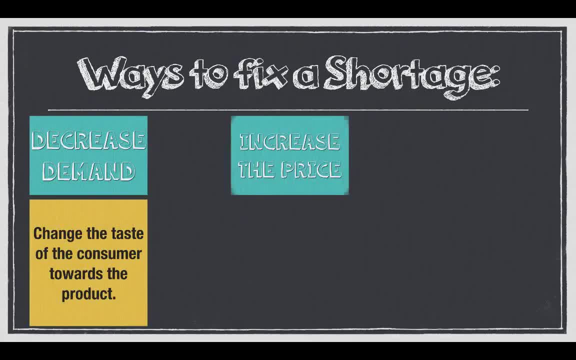 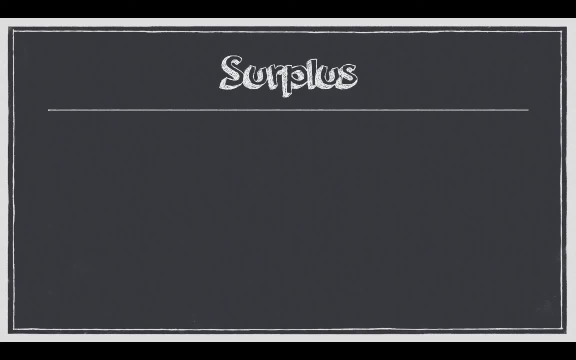 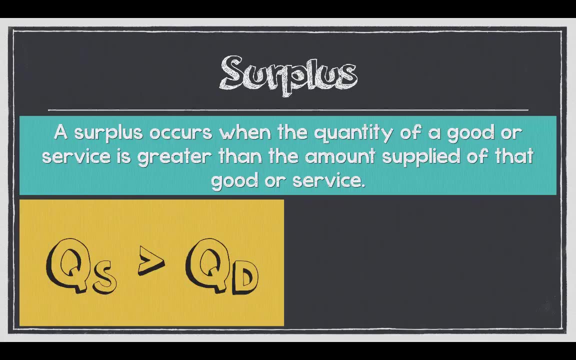 Ways to fix a shortage include decreased demand. so change the taste of the customer, increase the price, create a higher price and increase the amount supplied. maybe work more factory hours, or whatever it might be. We talk about surpluses. What we're talking about is we're talking about the quantity of a good or service that is greater than the quantity supplied. 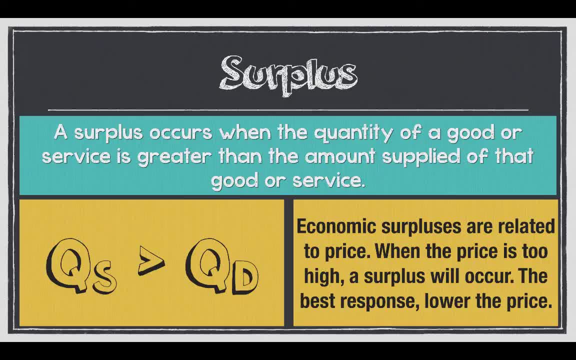 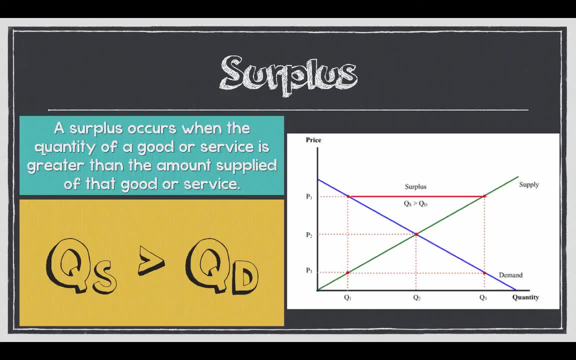 or is less than the quantity demanded. Quantity supplied is greater than the quantity demanded. Economic surpluses are related to price. When the price is too high, a surplus will occur. The best response is to lower our prices. Here's an example. 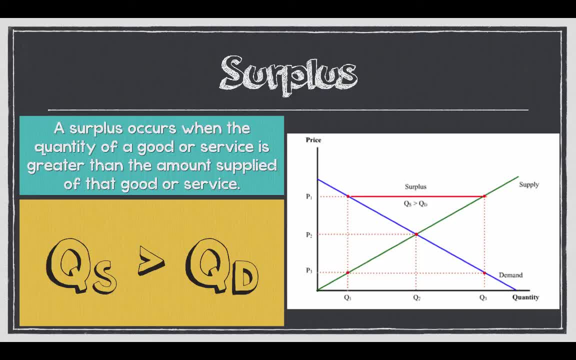 P1, we see a demand that is relatively low because of the highness of the price And we see a supply that is relatively high because of the highness of the price. So to find surpluses and shortages we rely upon what's known as the law of supply and the law of demand that we reviewed at the beginning of this lesson. 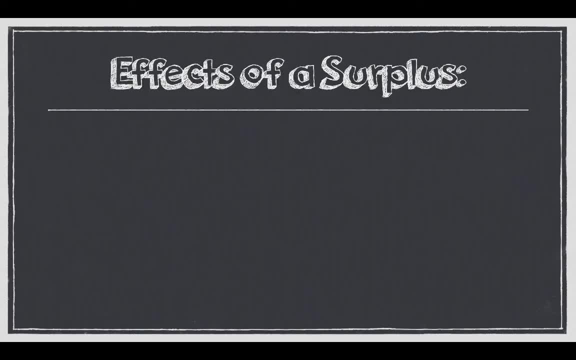 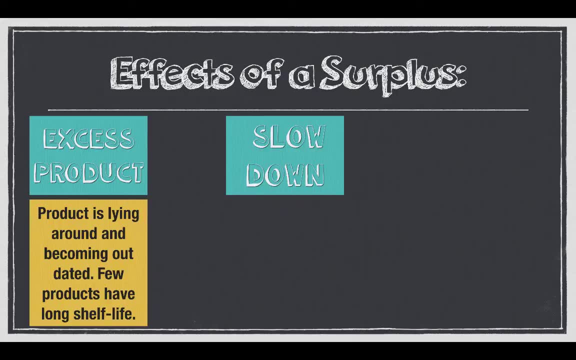 So what we see there is- we see that kind of taking shape, Now ways that we can fix this or the effects of it- is we have extra product lying around. You guys are going to read an article about corn and how we're just going to have piles of corn in the Midwest because we're producing too fast. 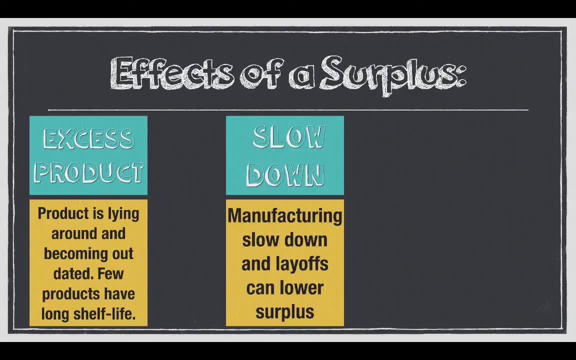 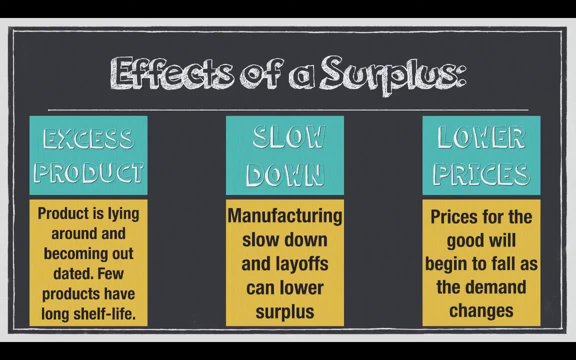 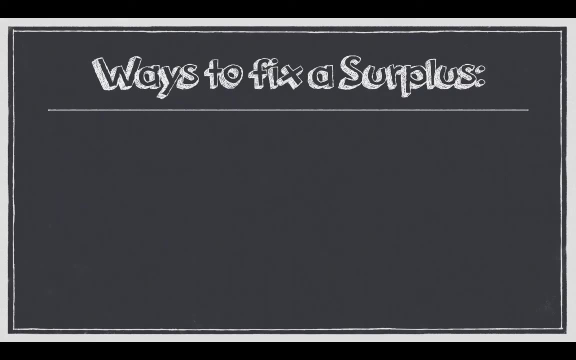 We may have to slow down, see an economic slowdown because we don't have enough people purchasing things might be a response. And then we see lower prices. Lower prices for good will begin to fall as the demand starts to change And we'll start to see that we are willing to purchase more at a lower price.